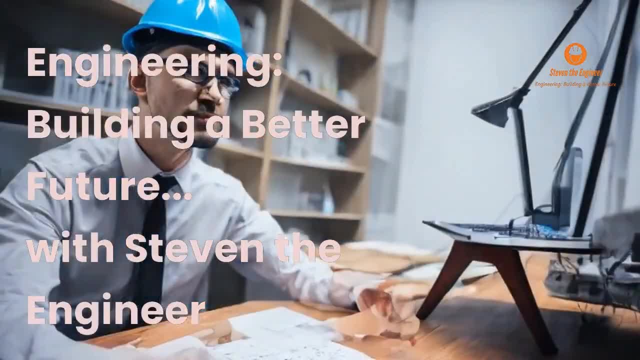 Engineering. Building a better future. With Stephen the engineer. What is geological engineering? At its core, it's a field that focuses on how the earth and its resources can be used to solve engineering problems. Geological engineers work in a wide variety of industries. From mining and energy extraction. To environmental management. And infrastructure development. They use their knowledge of the earth's geology. Minerals. And materials to help design and construct safe and effective engineering projects. In the energy sector, geological engineers help locate and extract oil. And natural gas using advanced exploration techniques. In infrastructure development, geological engineers play a crucial role in assessing the geology and soil properties of a site. Ensuring that structures are built safely and sustainably.